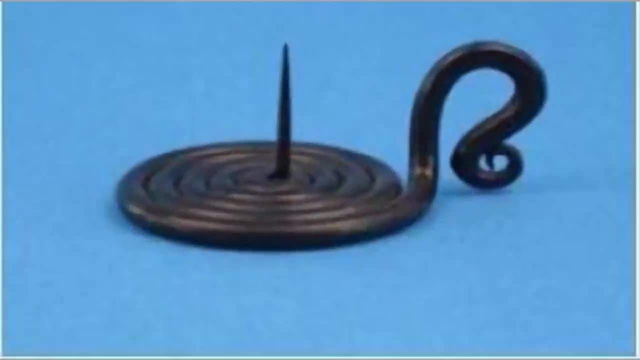 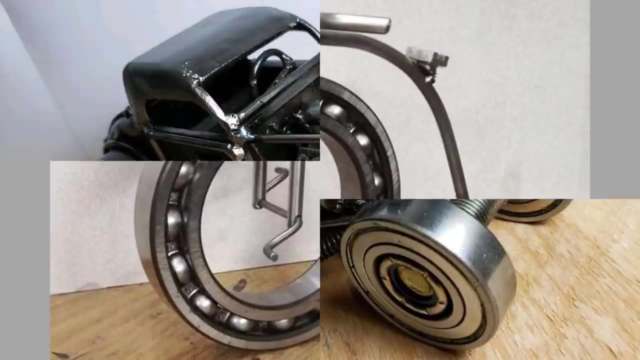 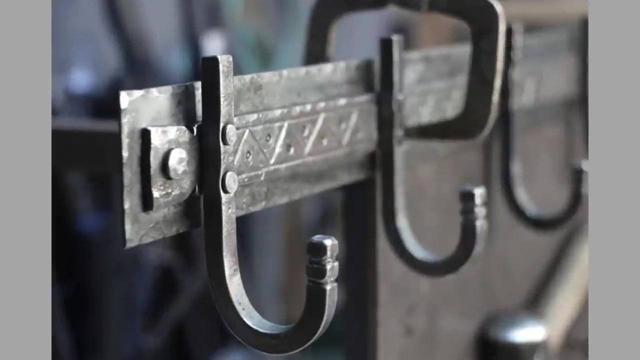 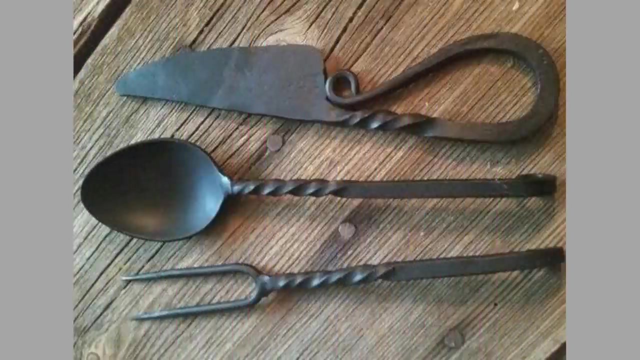 so that you will be the first one to be notified whenever we upload a new video. If you are already a subscribed member, please like and share this video so that it could reach a wide range of audience. There are several types of metals which could be used. 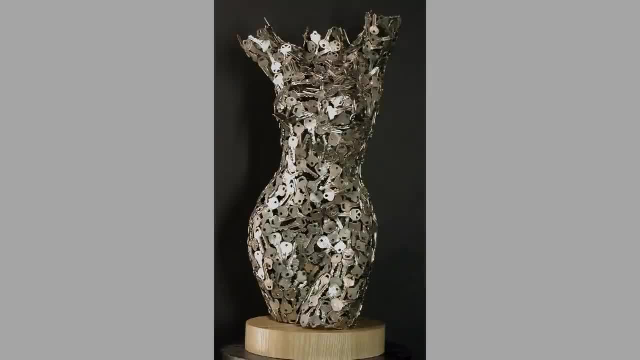 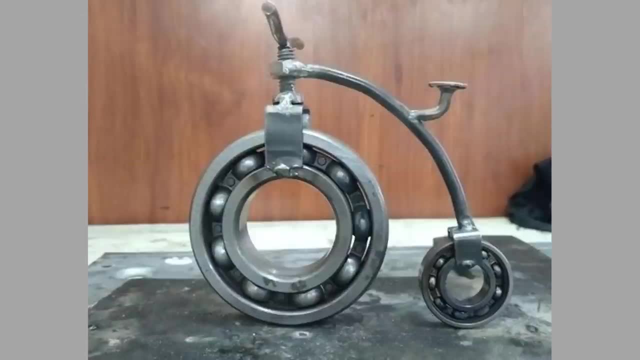 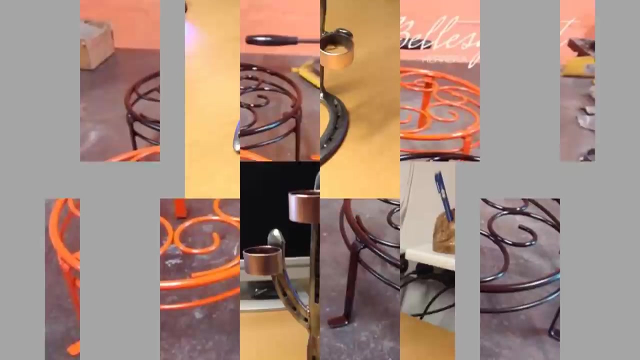 in the making of metal art and decor items. Let's have a look at some of these metals in the following sections. Iron Ore- Of all the known metals, iron is the most abundant of all and can be found in almost all elements. It is known to be a prized metal from ancient times. 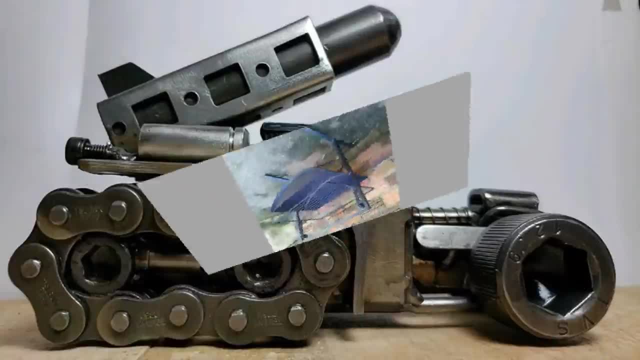 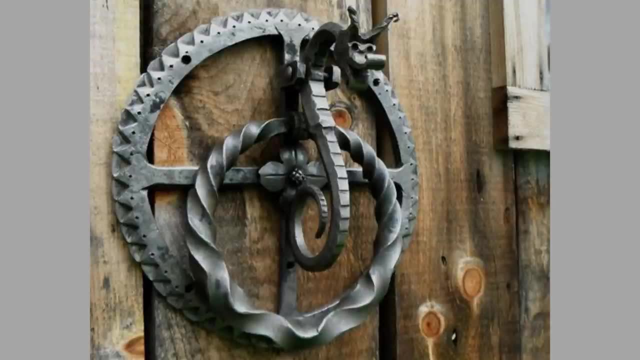 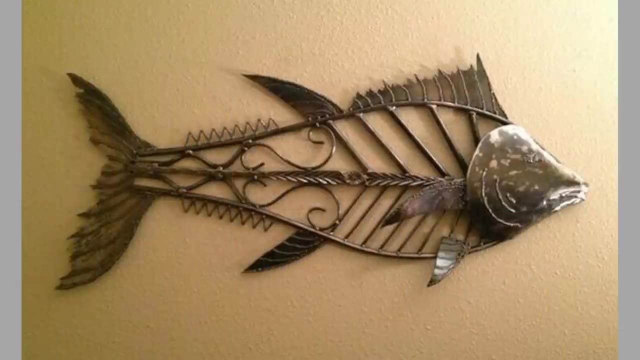 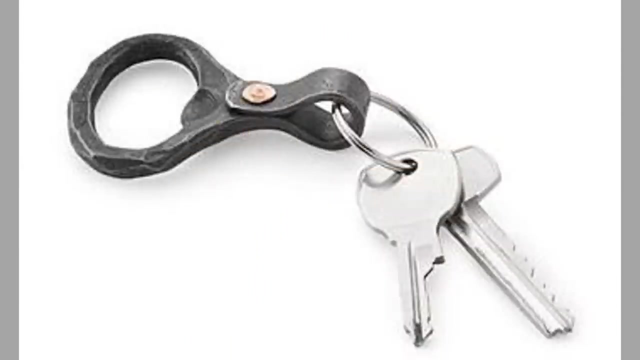 and iron objects have been discovered in Nineveh, Egypt, Roman Britain and ancient China. This metal isn't exactly pure, because it contains some silicon, sulfur, carbon and phosphorus, with the three principal varieties of commercial iron- cast iron, wrought iron and steel- containing various degrees of carbon compounds. 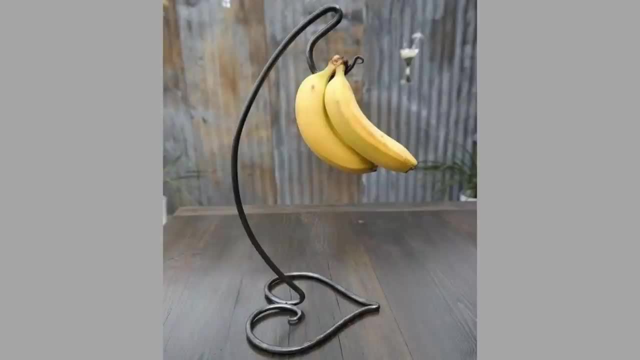 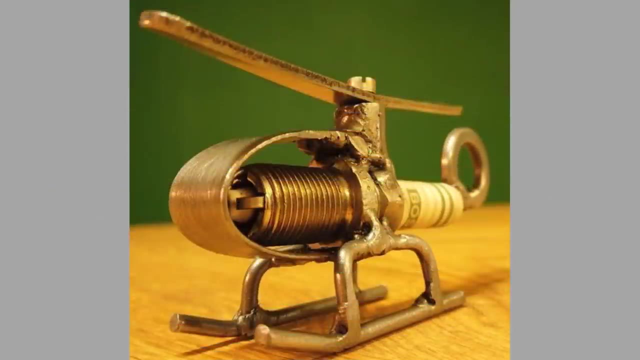 Old artwork and sculptures, including other iron objects, are likely to rust when they get exposed to damp air, moisture or water. However, because iron ore is prone to rust, it can be prevented when coated with non-oxidizing materials like tin. 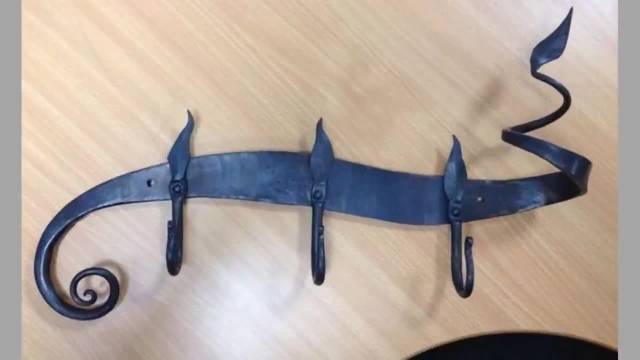 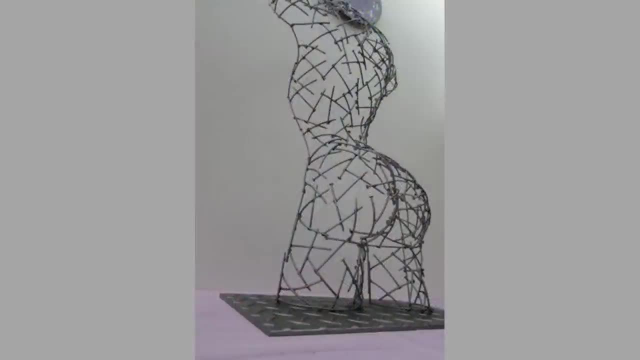 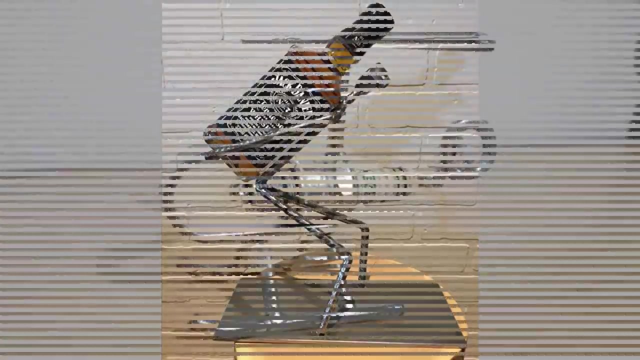 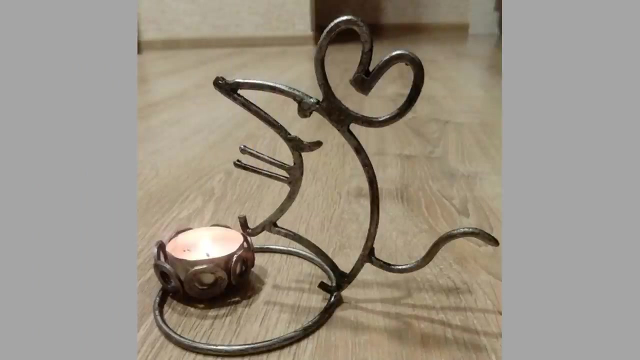 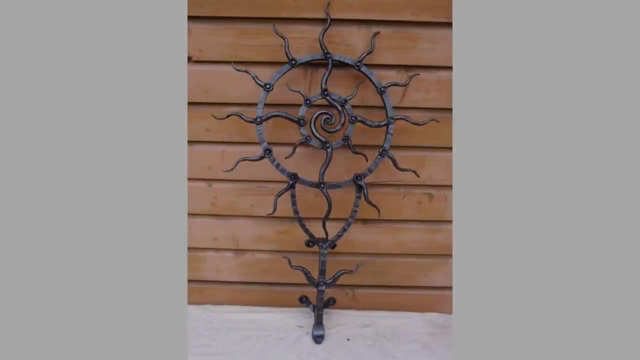 brass or zinc. Iron is made into personal adornments, hand tools, cooking pots, garden sculptures and drinking vessels, along with ornamentation of weaponry, horse tags, boats and other functional items. The amount of carbon in cast iron wrought iron and steel. 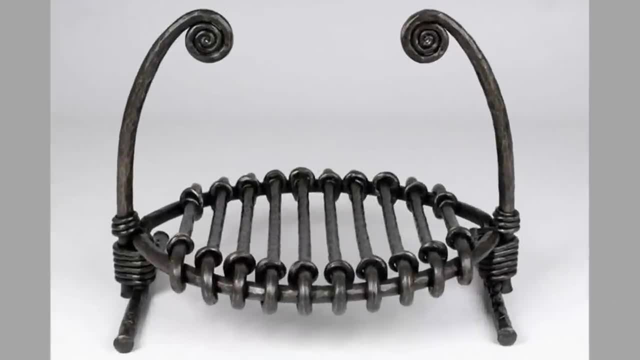 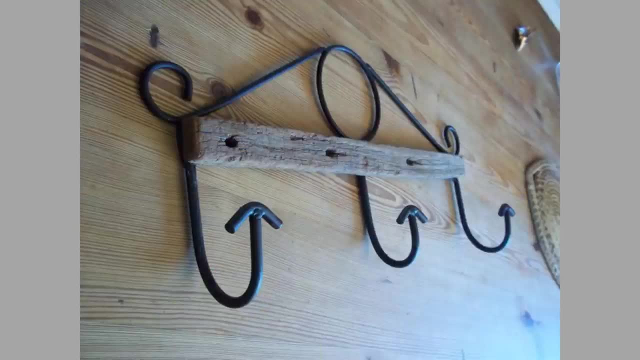 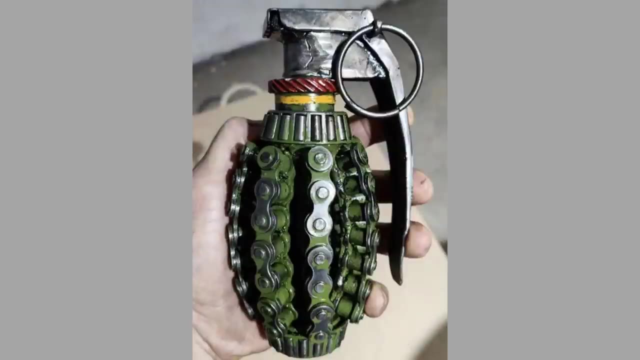 is what determines their character, strengths and working qualities. Wrought iron contains the least amount of carbon, while cast iron contains the most. From larger-than-life sculptures to irresistibly petite decorations and art forms, all the different types of iron artwork are made from one of the following: 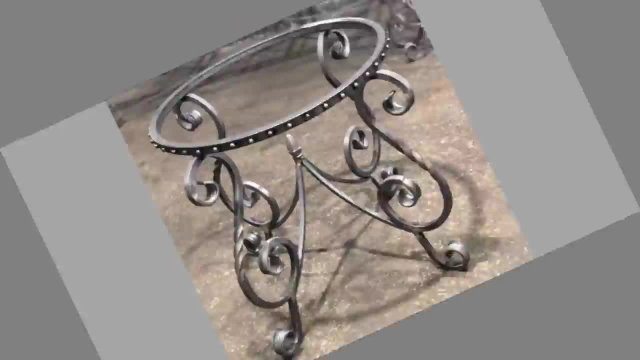 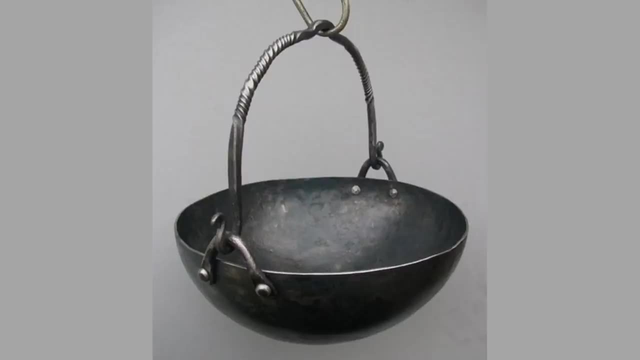 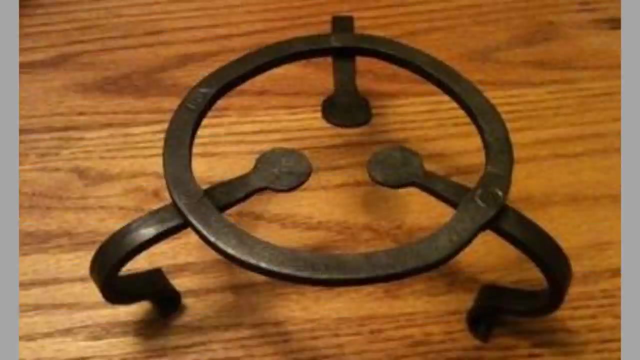 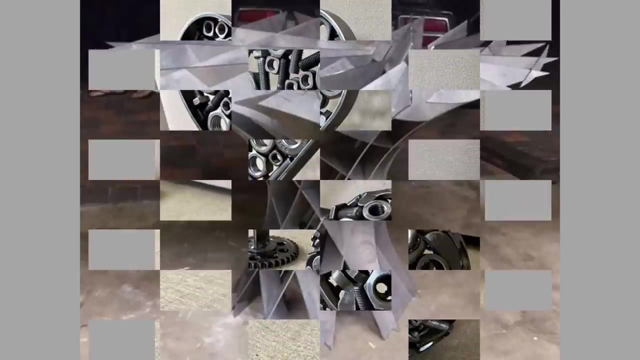 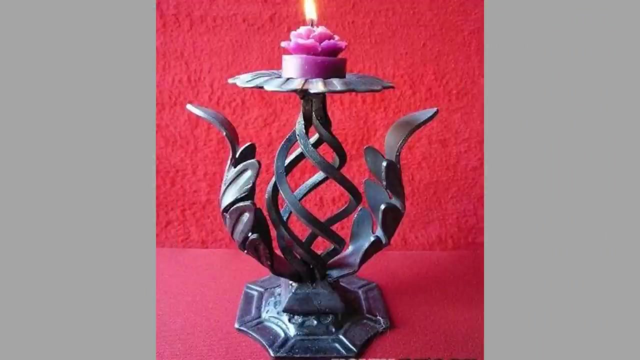 cast iron steel, stainless steel and wrought iron Cast Iron. It contains a good amount of carbon which gives it a brittle quality. It cracks easily if hit. Art is extremely coarse and cannot be stretched or bent. Cast iron isn't really used in the decorative art because of its roughness. 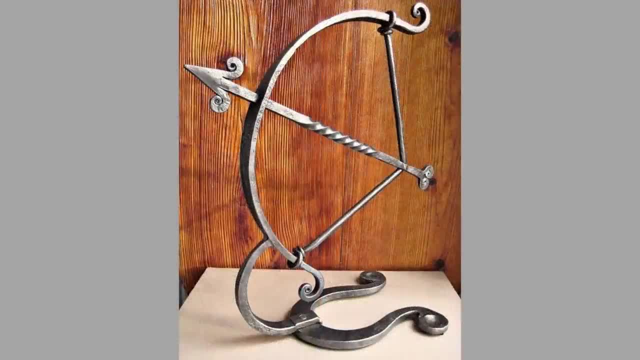 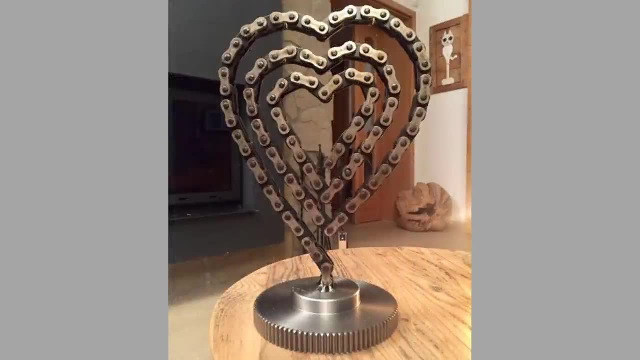 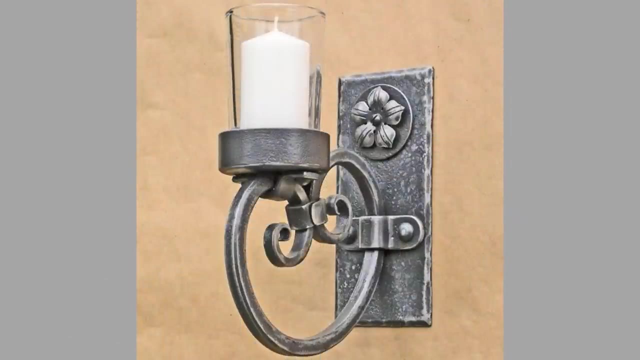 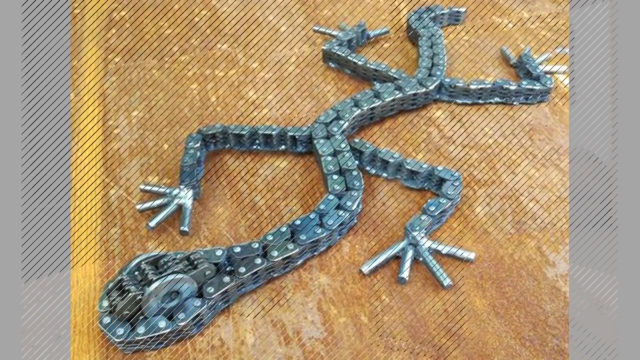 but is mainly used for ornamental firebox and facings, fireplace accessories and traditional stoves. Steel Steel's hardness is the midway between wrought iron and cast iron, so it possesses characteristics of both. It has a finer grade and is lighter and malleable if exposed to very high temperatures. 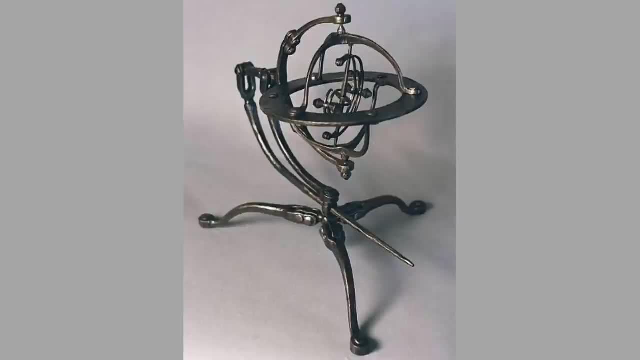 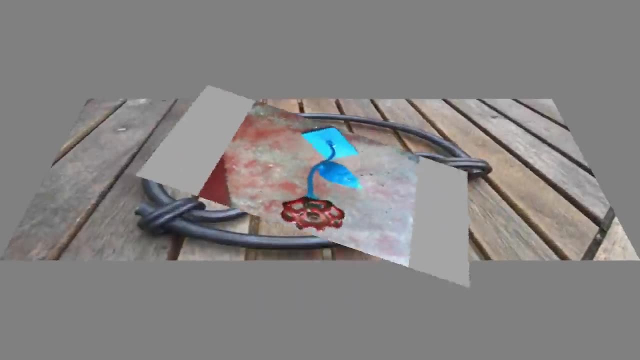 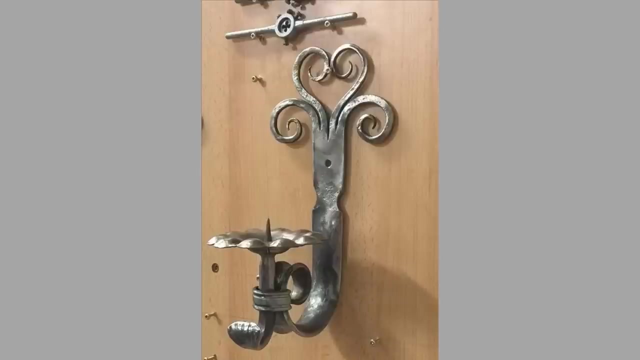 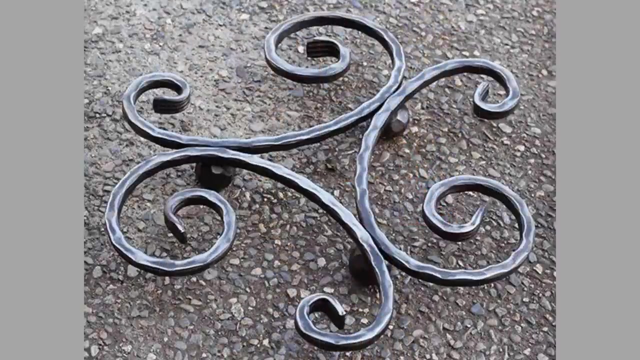 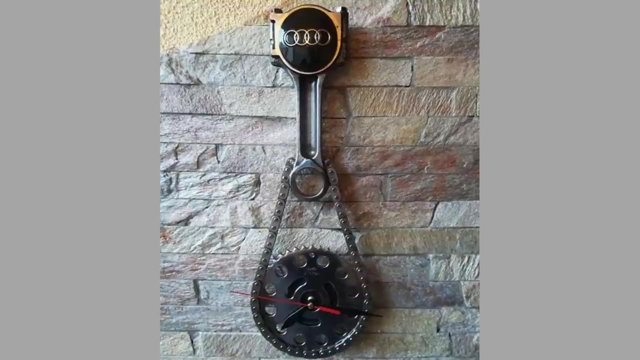 With sudden cold temperatures it becomes extremely hard. Steel has a shine and toughness. Though it is used majorly for structural works and reinforcement materials, it is also used for contemporary artwork and sculptures. Stainless Steel Alloying chromium with steel helps to prevent it from rusting and retain its luster. 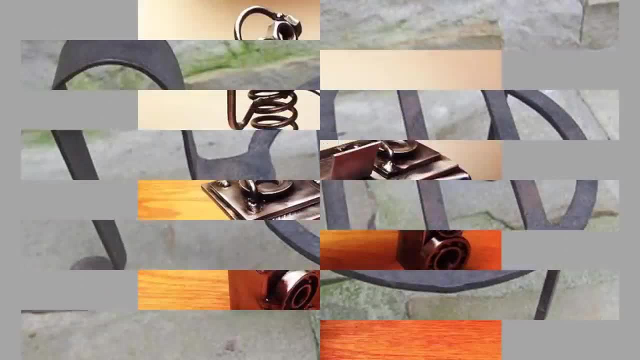 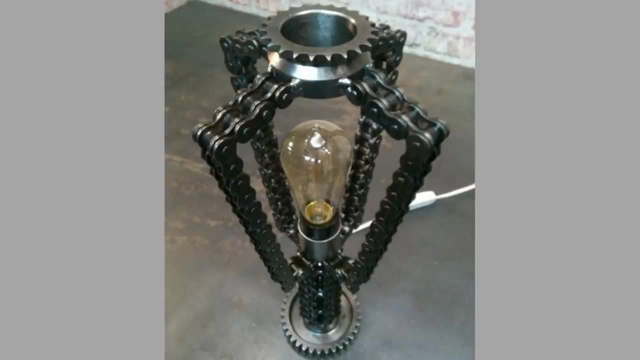 and stainless steel is used for this purpose. Stainless steel is alloyed with 10% to 20% of chromium. Its luster, non-rusting qualities and its beauty make it suitable for exquisite cutlery, staircase railings, decorative hardware and jewelry. 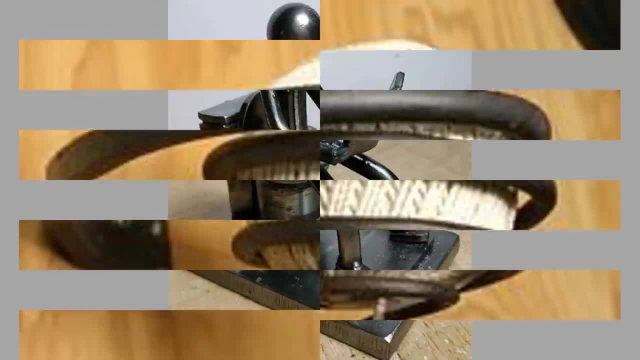 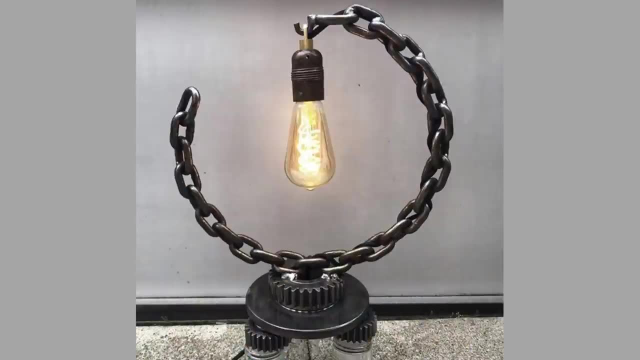 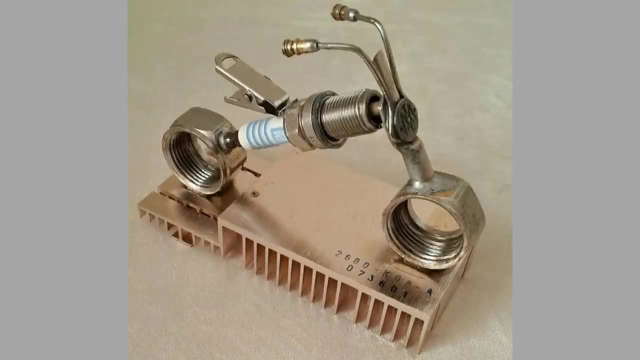 Wrought iron. Wrought iron has fewer carbon impurities than cast iron and is softer in nature. It is easily rolled into plates, hammered into bars and drawn into wires. Its malleability allows it to bend into any shape or form. Wrought iron items can be painted with brass. 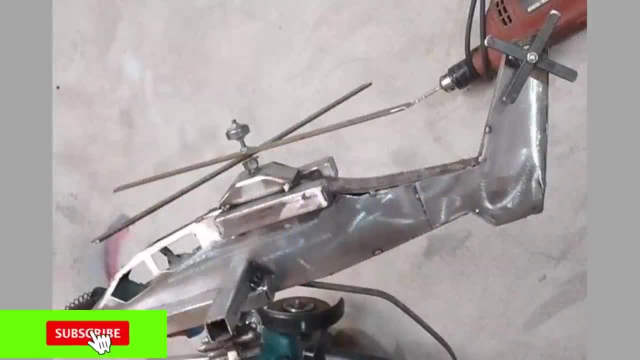 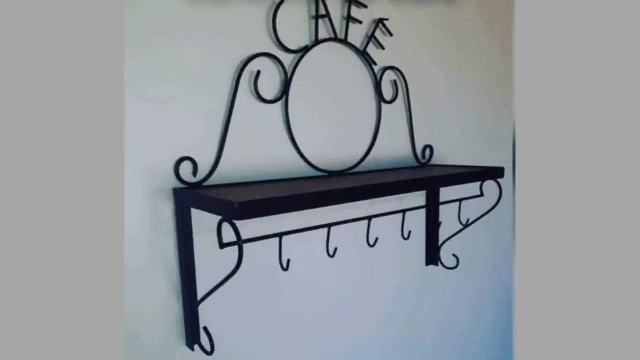 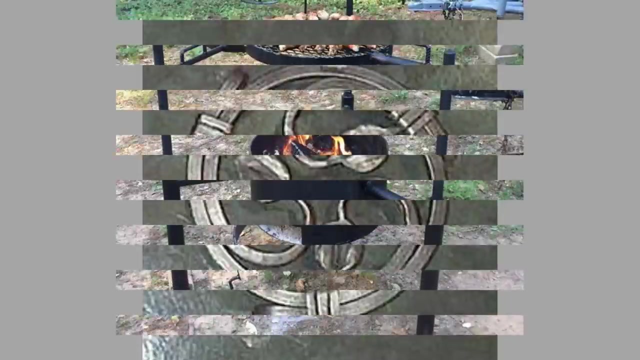 and various thicknesses of the iron can be used for cheaper hardware: braces and brackets, Garden furniture, outdoor ornaments and garden sculptures, fireplace linings, railings and balustrades, grills and affordability. moderately light fittings. 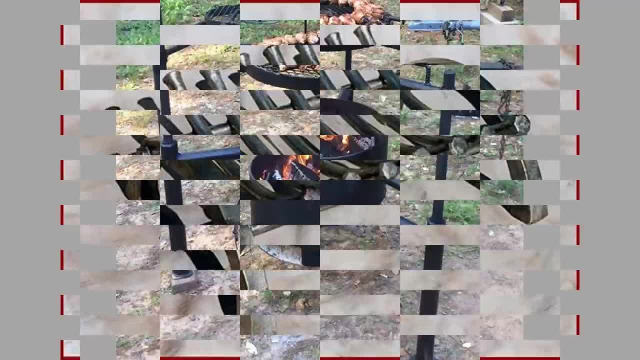 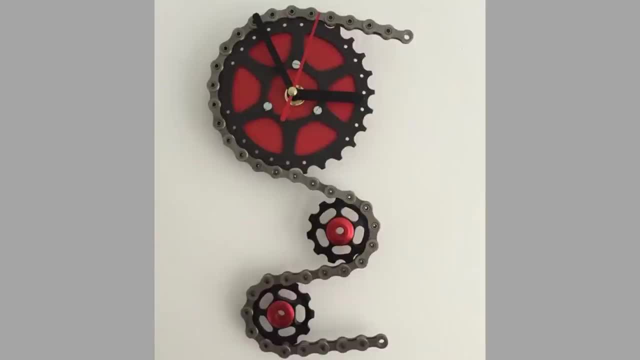 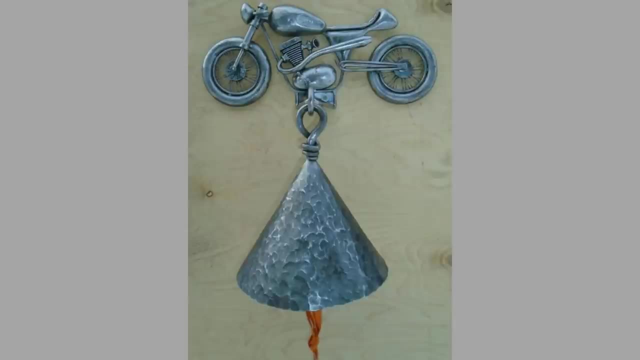 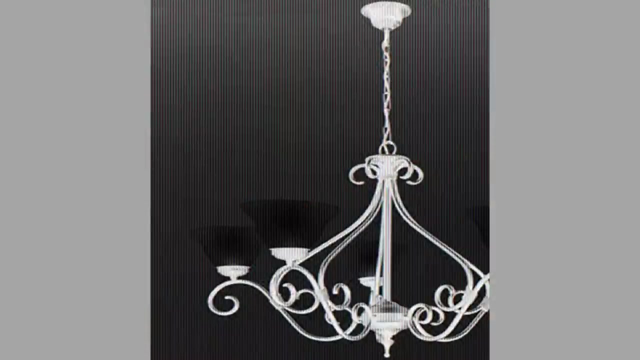 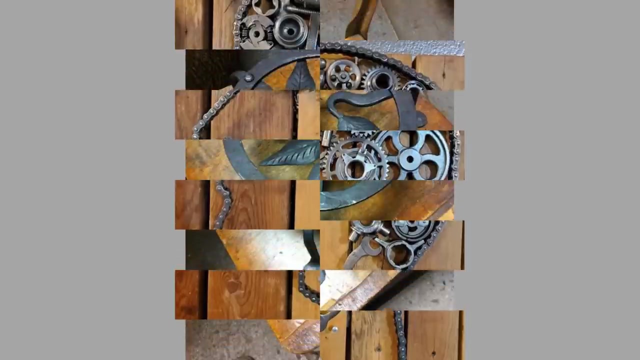 2. Thin. Thin is majorly used for metal wall artworks, plagues, floral sculptures, hanging ornaments, thin-walled signs, busvariets, decorativeациads, water vessels, ornate vases, candlesticks. thin foil art tin in all forms have been used for recycled art, with some of the most awesome. 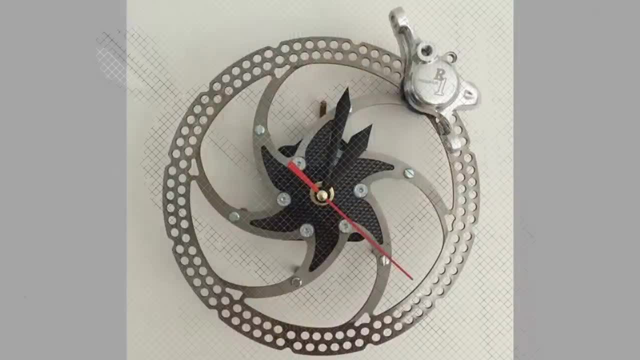 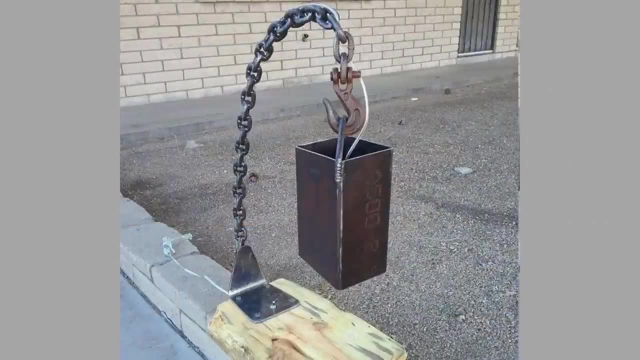 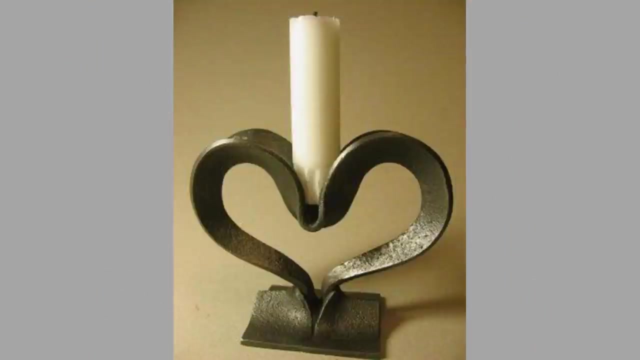 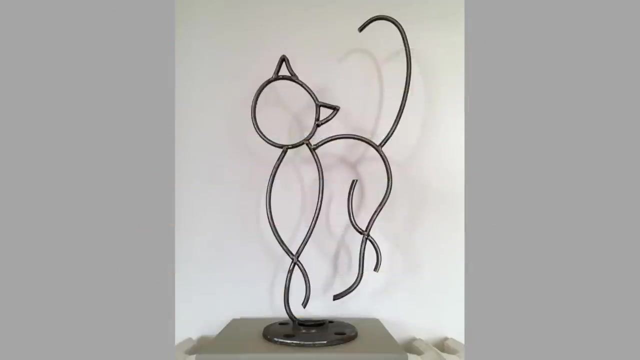 metal art format. this way, recyclable tin materials include bottle tops, sweet things, food cones and the like. one of the least known but beautiful expressions of metal art are the thin artworks first produced in mexico around the 16th century because tin was not only available and inexpensive. 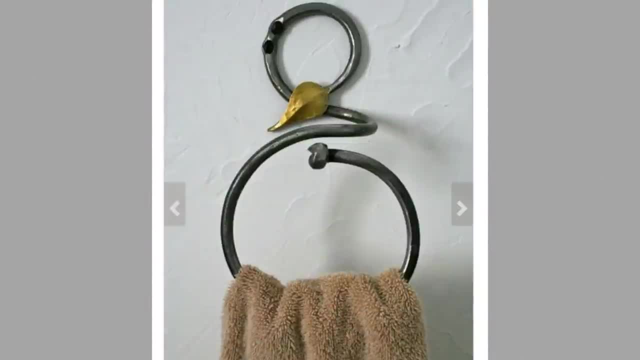 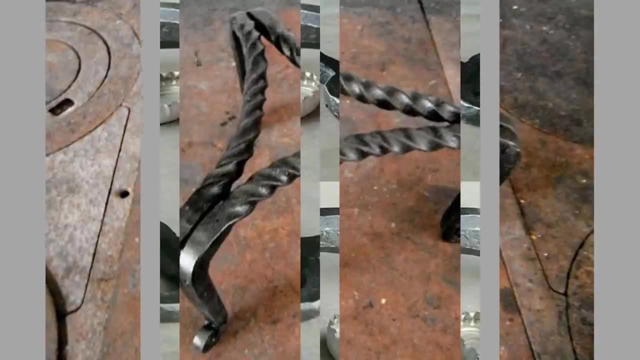 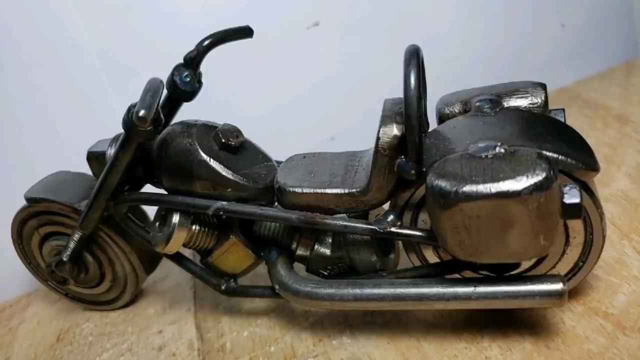 it was light and malleable. this made it easy to shape, crimp, stamp, punch and cut into a wide variety of decorative and functional artwork and paint in pleasant colors. thin, shiny surface that looks similar to silver is what likely contributes to it is appeal for making art objects and sculptures. 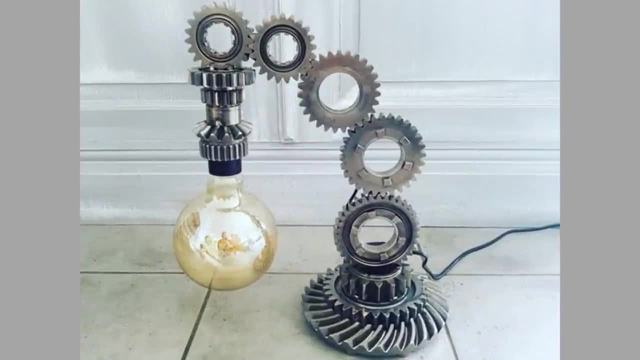 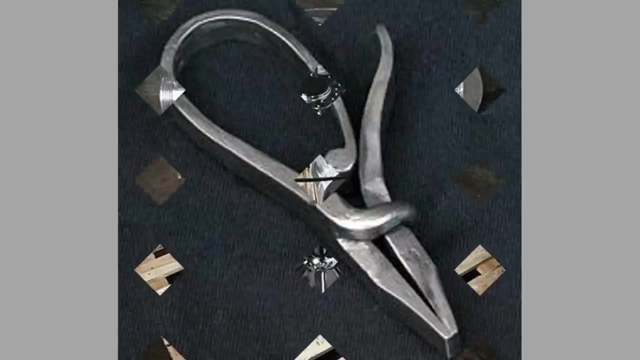 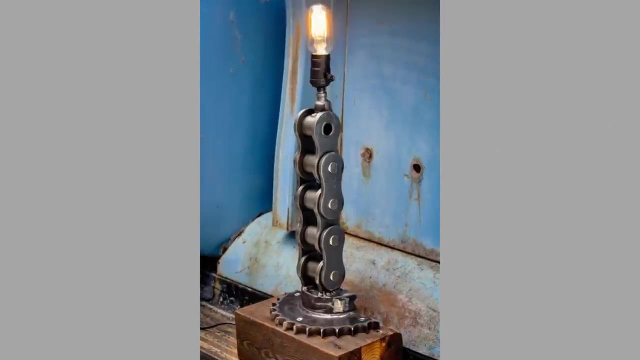 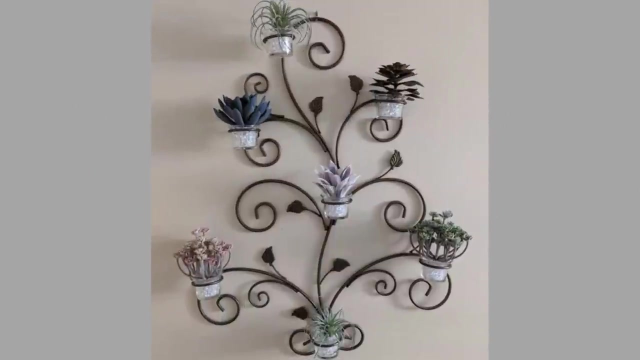 regardless of it is tendency to rust. number three: copper. copper is a metal that is found in its pure state, just as silver, gold and thin, and predates iron in terms of its use. according to the history of art, most nations used copper extensively as materials to make coins, weapons, statues, deco and household. 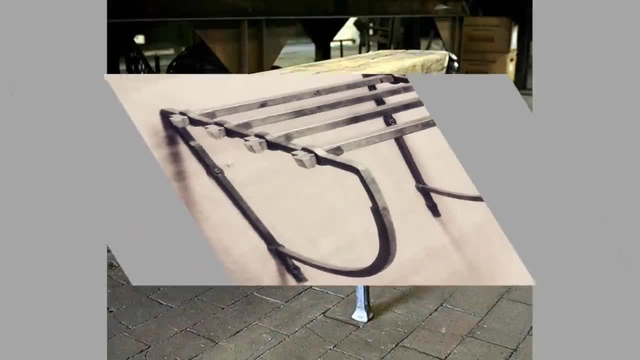 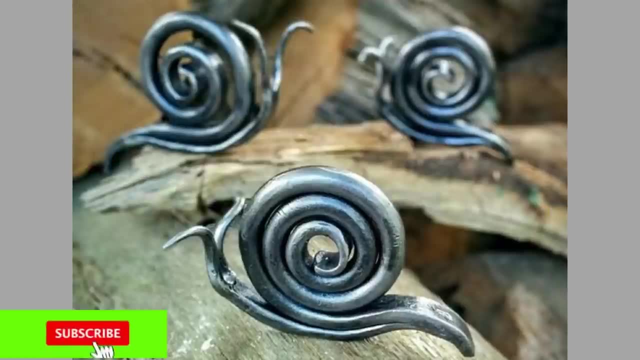 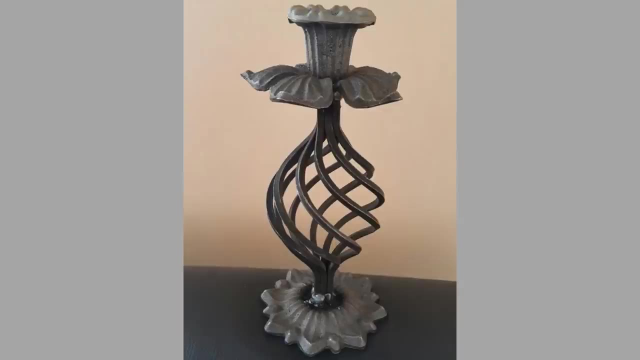 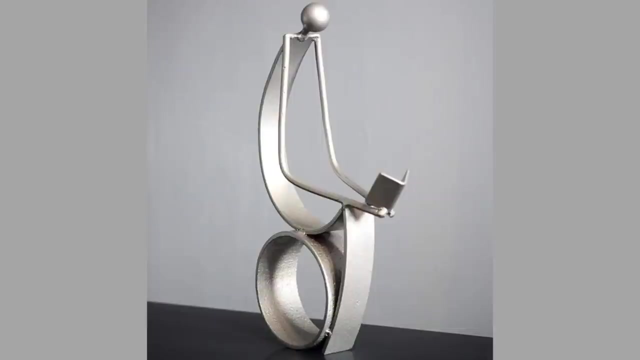 items. it is also claims that ancient egyptians used corporate chisels hardened by a now no unknown process to cut their granite. this metal is used rolls for decorative and industrial art and is favored for its strengths, durability and its workability. that is with which corporate can be molded. it can be hammered or cast. 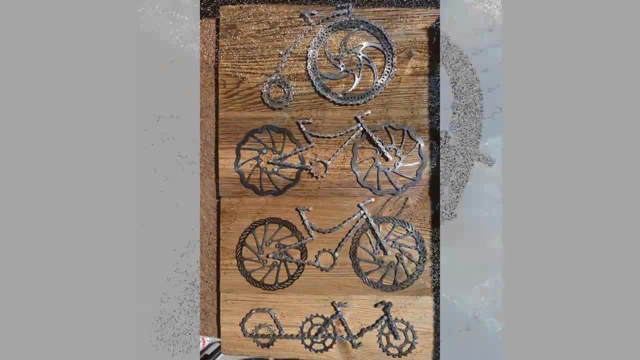 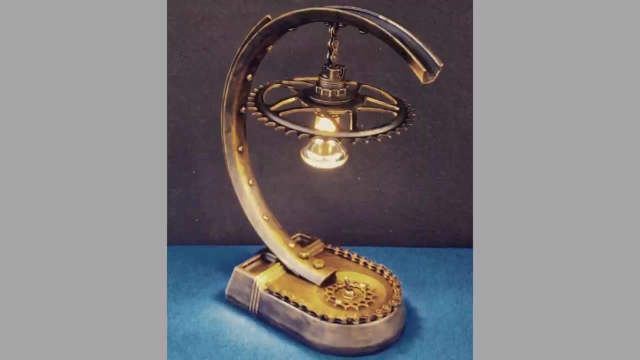 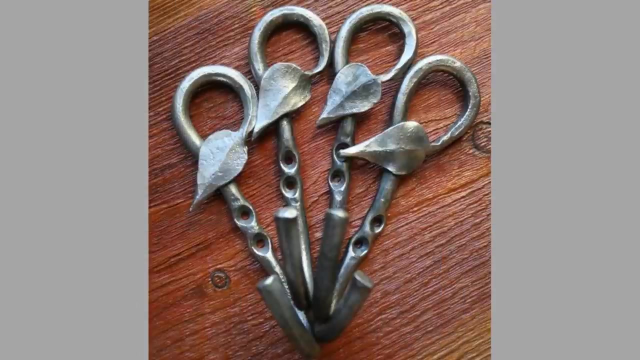 into any desired shape or form, makes it a useful and great metal to use for the following hardware: sculpture works, wall art, statues, table ornaments, vases and urns, display pedestals, lighting fixtures, screens, grills, kitchen utensils, ethnic jewelry and cloaks. 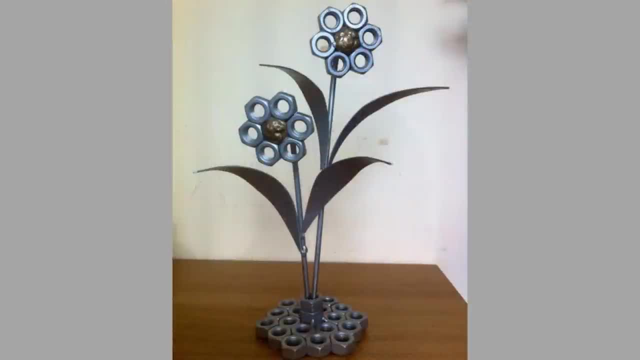 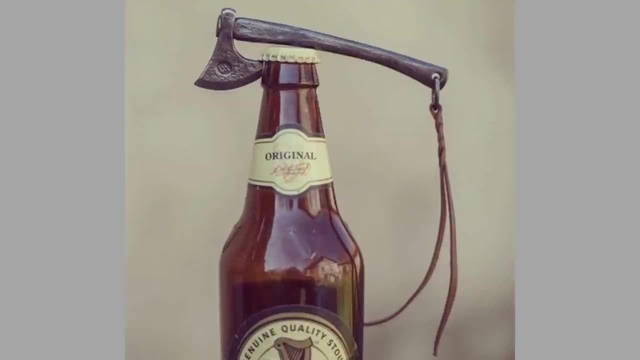 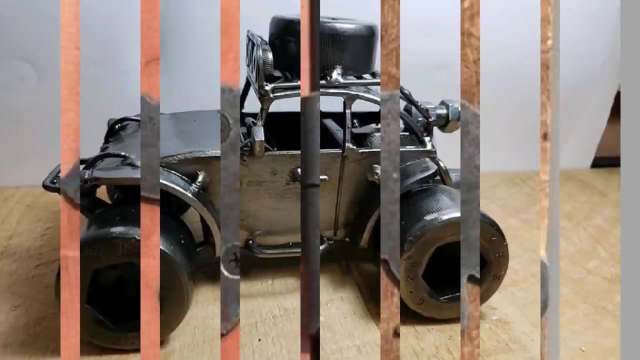 Jewelers combine copper with silver or gold to harden them for jewelry making. Copper is also alloyed with nickel and zinc to make beautiful pieces of German silver. Because copper is very durable, it is used extensively for the production of small ornamental objects and for structural objects that can't endure excessive strain. 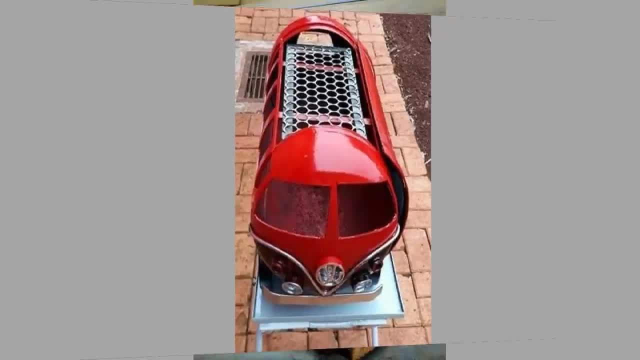 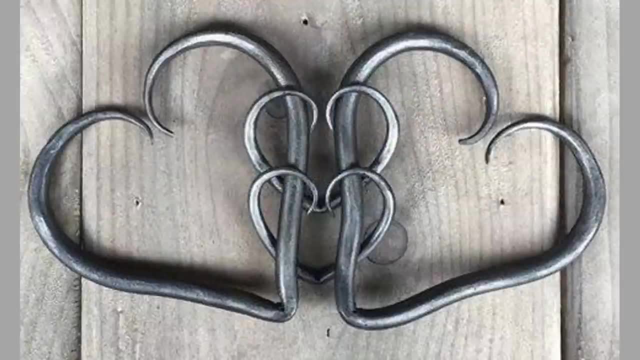 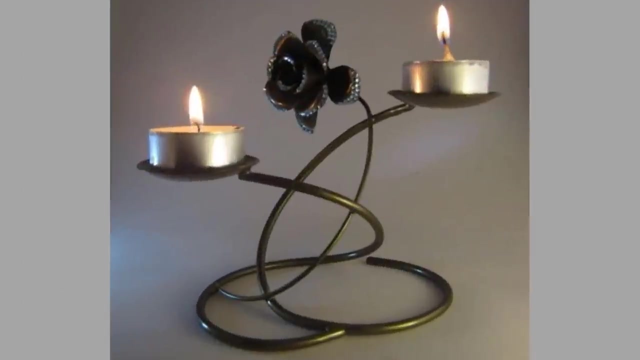 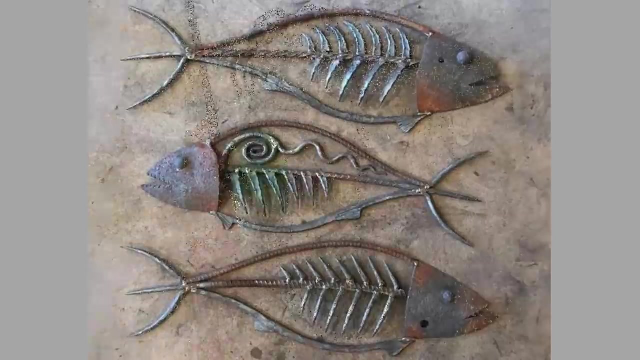 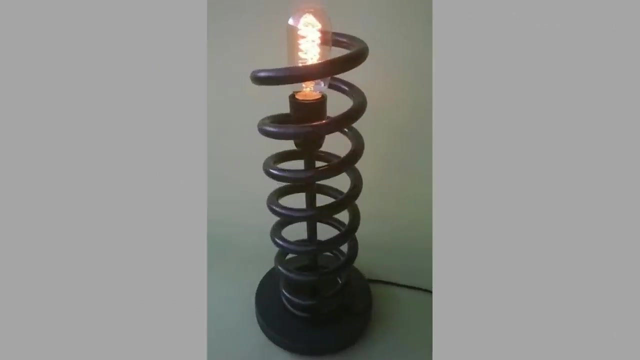 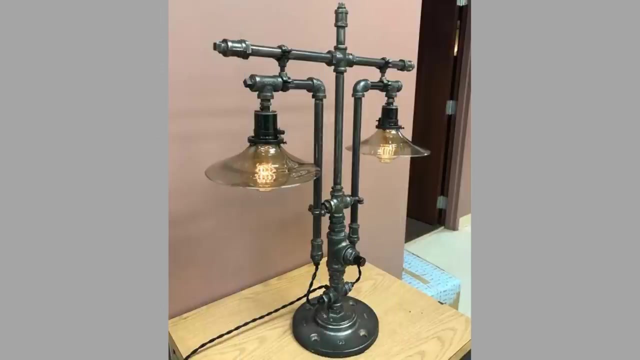 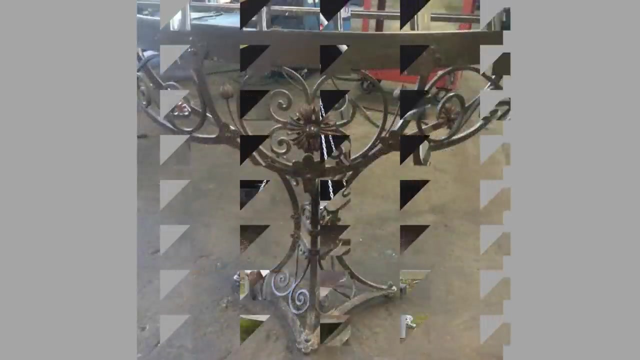 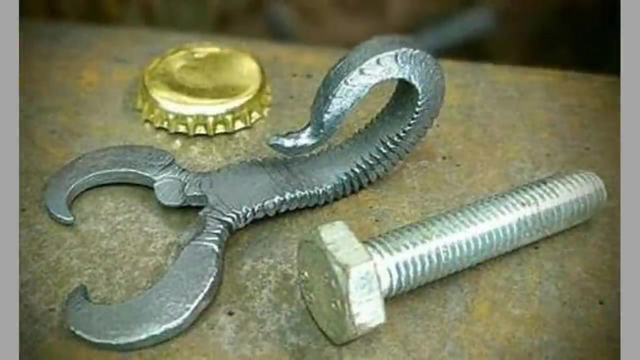 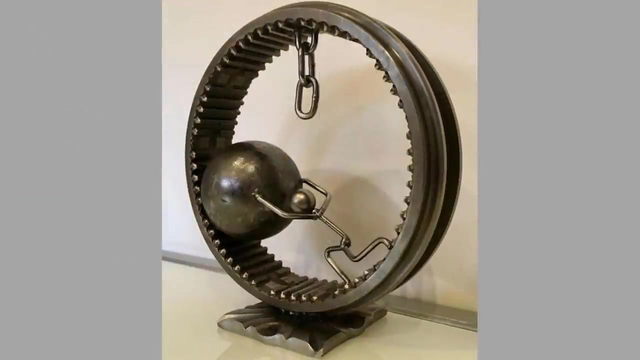 The silver color on the glass is also famous for the fact that the silver and the copper are well-tuned. The silver color on a work surface is also made with silver and silver. Thank you for watching. See you next time. Thank you.